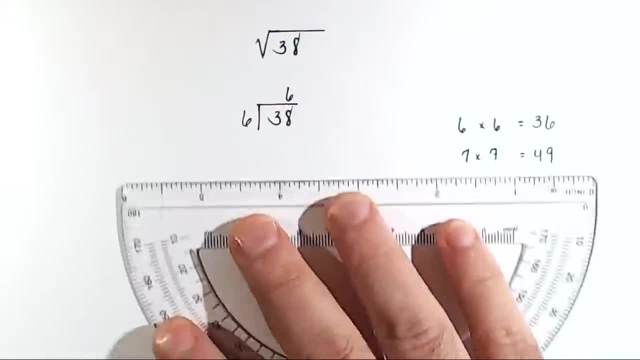 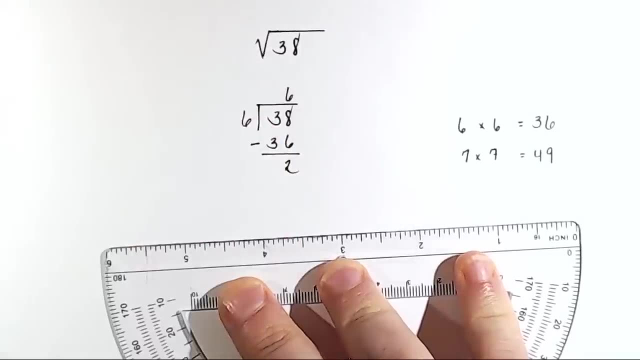 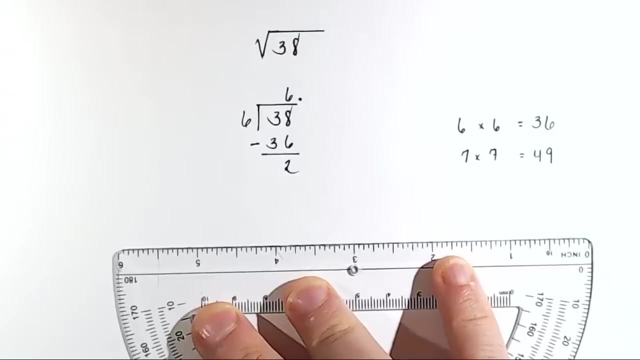 And 38 divided by six is six. Six times six is thirty-six, And we're left with a remainder of two. And here's the cool part. This is where it differs from division. on how you do this, Put a dot, All right. 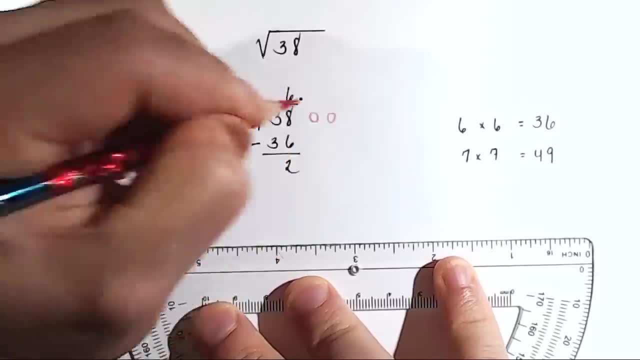 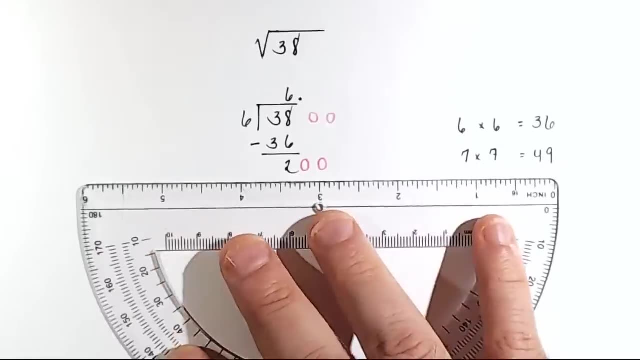 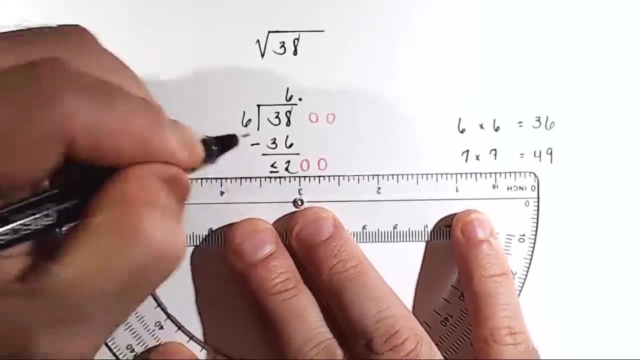 And now we're going to invent and bring down two zeros. All right, Set this template up just like I'm showing you. Next to 200. down here we will write a less than or equal to symbol, And to the left of that symbol we'll put a line. 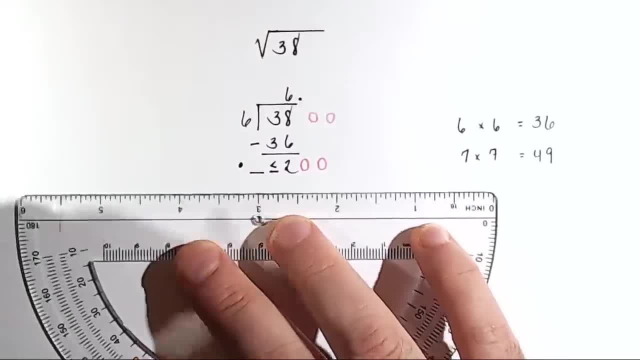 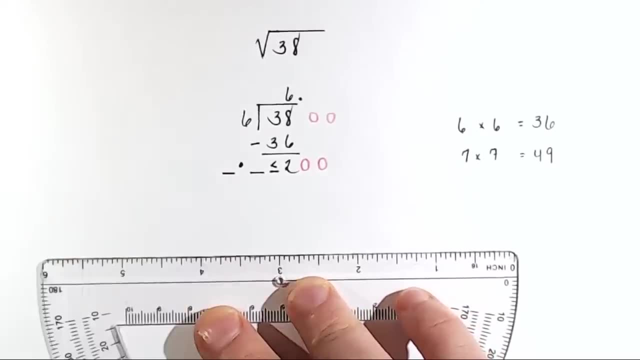 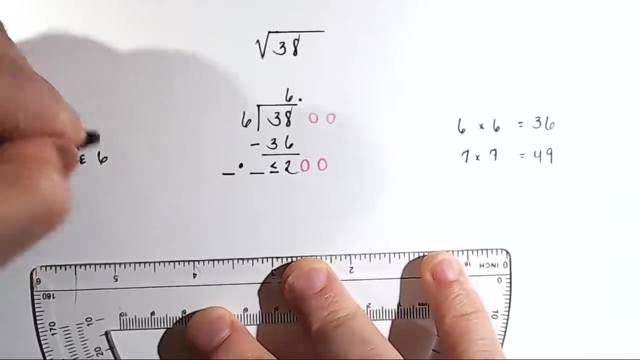 To the left of that line we'll put multiplication symbol. To the left of that symbol we'll put another line, And then, right here in this space, we need to double six. Six times two is twelve, So this is one two. 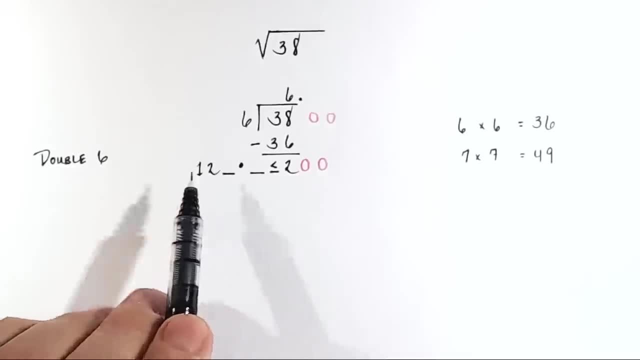 What we're looking for here is now a three-digit number whose last digit goes here. It's better to just see it happen, All right. So what we're looking for here is a three-digit number whose last digit goes here, All right. 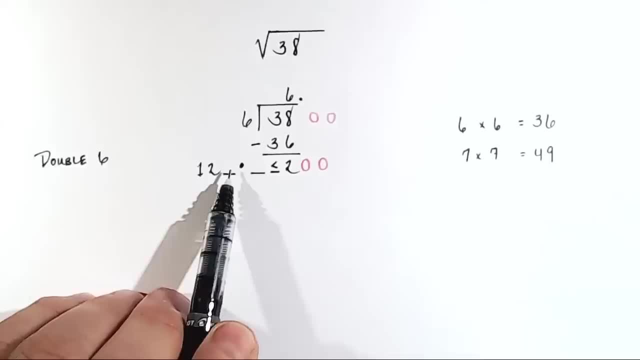 So what we're looking for here is a three-digit number whose last digit goes here, And what we're looking for is a three-digit number whose last digit can be placed here, And when you multiply that three-digit number by that last digit, you get a number that is less than or equal to 200.. 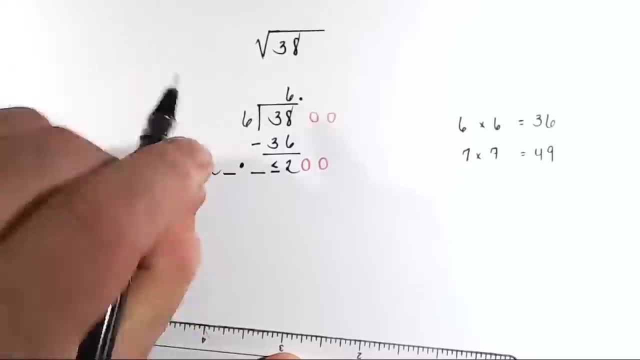 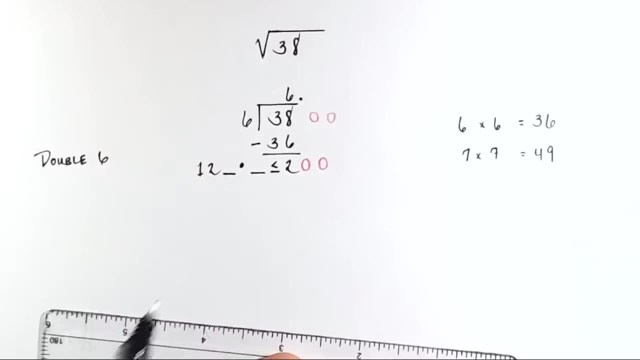 Well, it's just one, All right, Because if you did 122 times two, you would get a number that was bigger than 200. So it's 121 times one. Okay, 121 times one is 121.. Put that here. 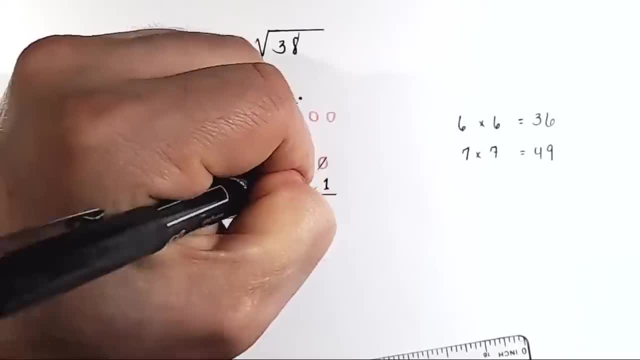 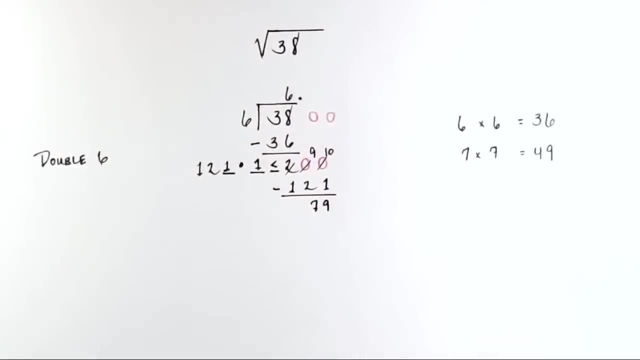 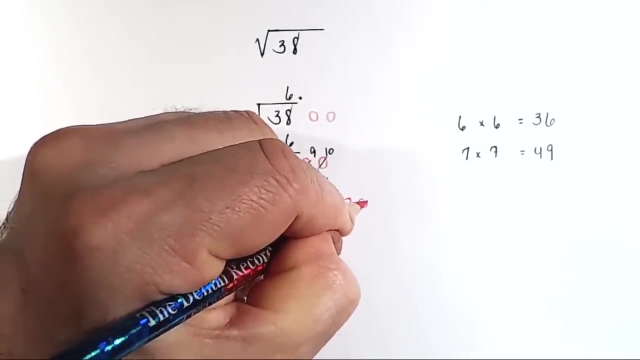 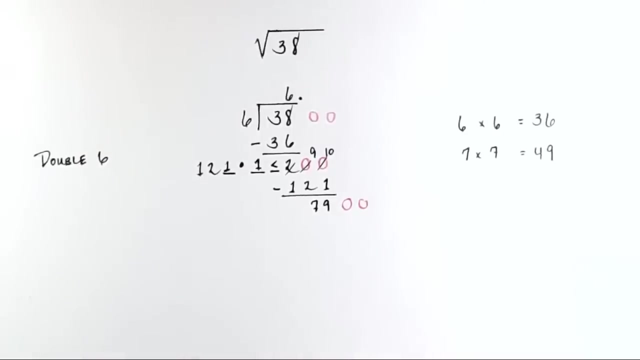 And now perform the subtraction: Ten minus one is nine. Nine minus two is seven, So now we're looking at 79.. And we will bring down two more zeros. So our next step is to evaluate up to 7,900.. But we have accomplished something awesome. 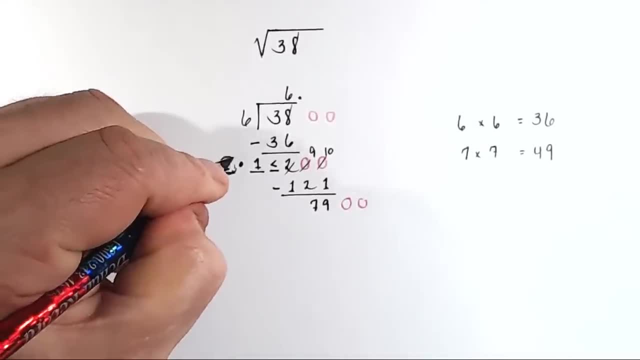 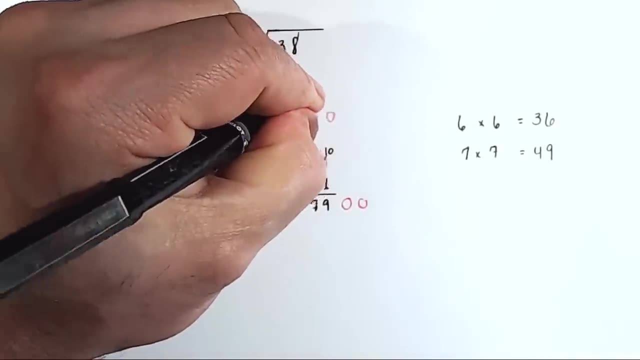 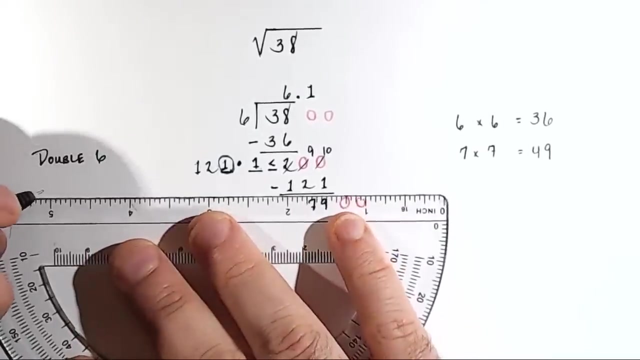 This number right here, one is the tenths place of the approximated square root, So we'll go in here and put 6.1.. Here's the trick: You've got 6.1, and I want to remove the decimal place. 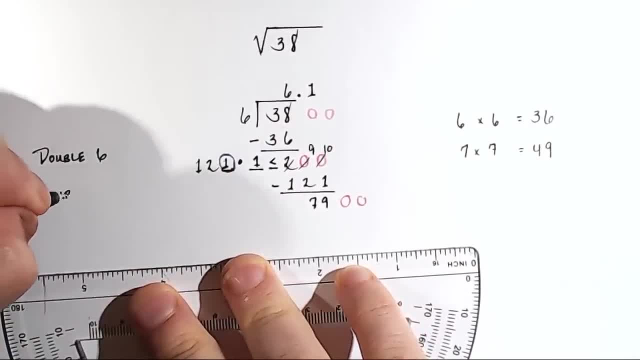 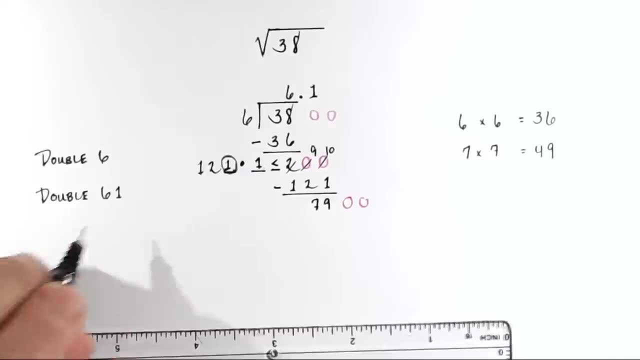 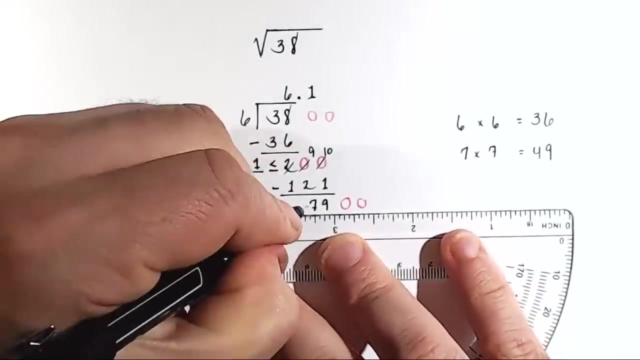 So we're going to double 61. So we'll do here: What is the double of 61?? Well, that would be 61 times 2.. So that is 2 and 12.. So here's where I'm going to place my less than or equal to symbol, right here. 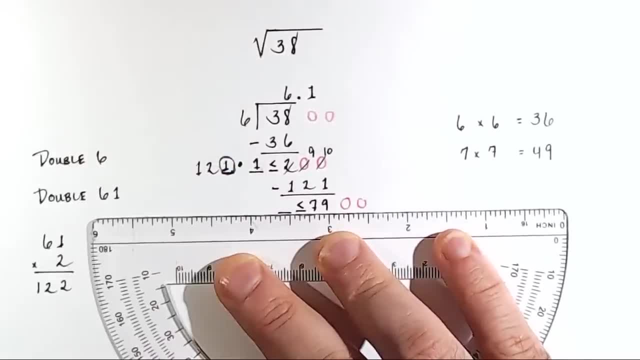 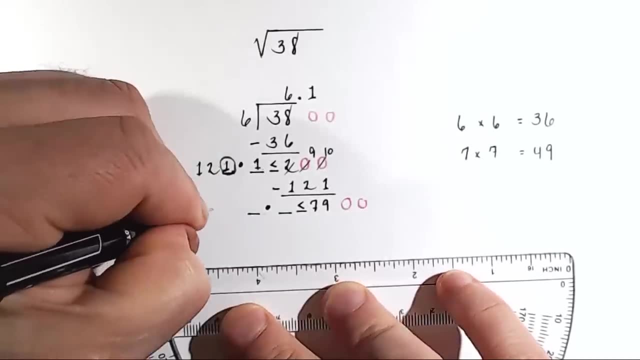 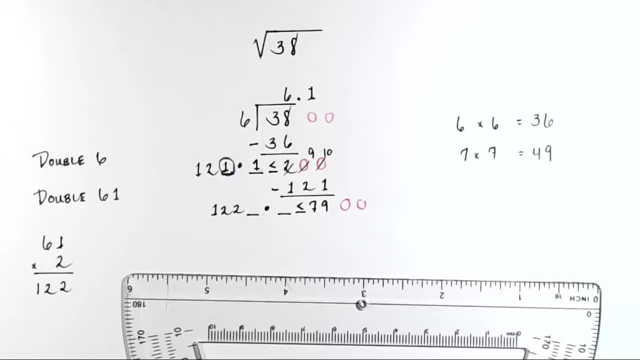 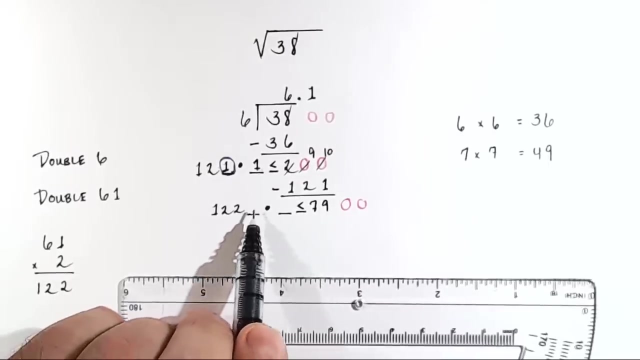 And then a little line, Multiplication symbol, little line, And then to the left of that I'll write 122.. Okay, What is the next step? The next step is to find a whole number that I can tack on to the end. 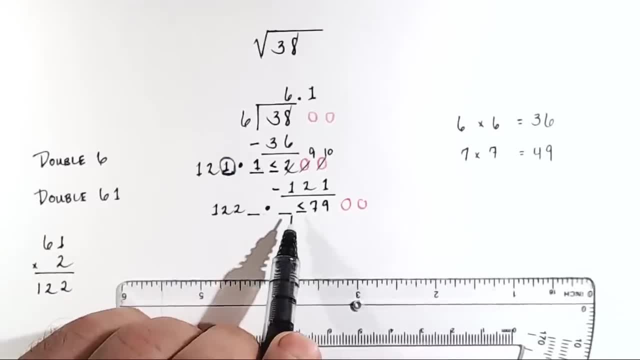 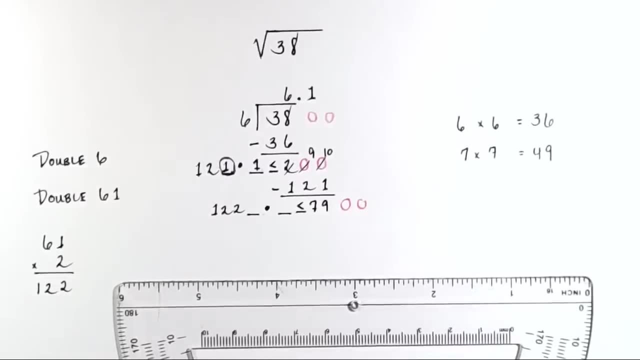 making this a four-digit number, And then, whatever that whole number is, I'm going to multiply it, this four-digit number, by that whole number, terminating one's place digit that I've found, And when I multiply it together it's got to be less than or equal to 79.. 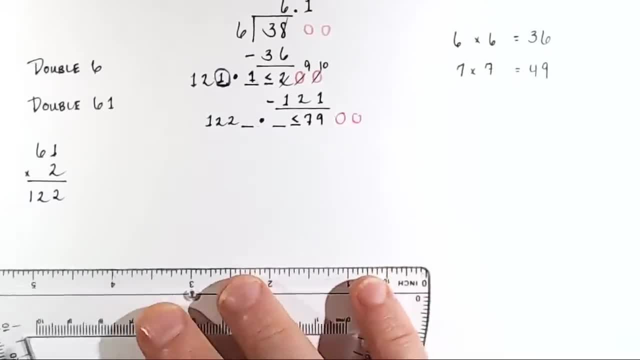 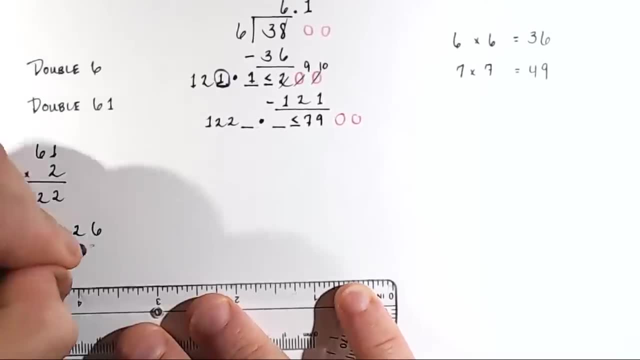 All right, So in this example we'll try 6.. Before we put it, let's try it: 1, 2, 2,, 6 times 6.. Let's see what that is. 6 times 6 is 36.. 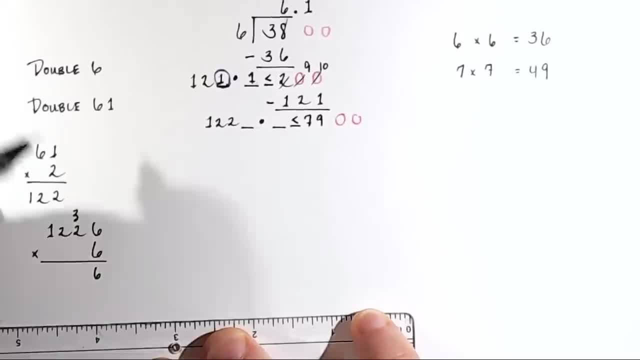 Carry the 3.. 6 times 2 is 12, plus 3 is 15.. Carry the 1. 6 times 2 is 12, plus 1 is 13.. Carry the 1. 6 times 1 is 6, plus 1 is 7.. 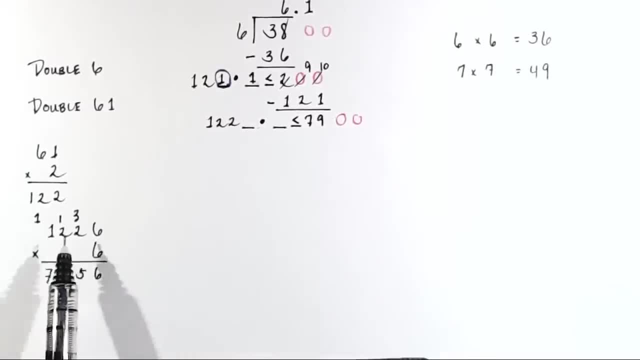 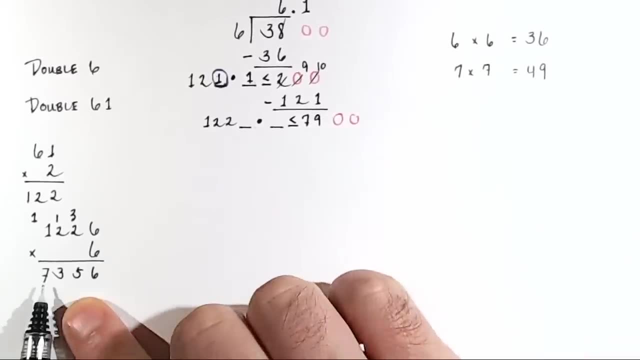 All right. So you see here we couldn't do 1,, 2,, 2,, 7 times 7, because it would be bigger than 7,900.. This is as close as we're going to get, So we'll go up here and put a 6 here. 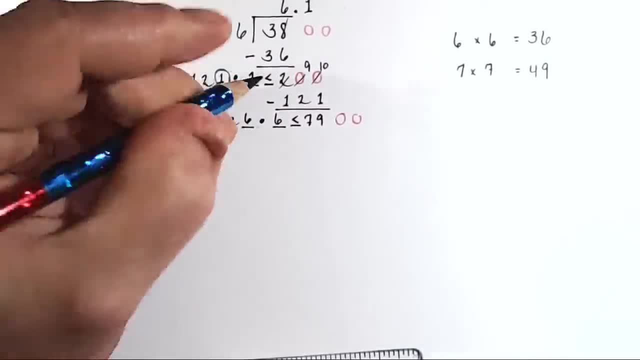 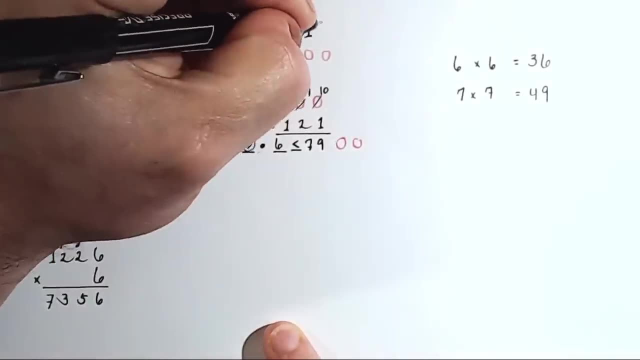 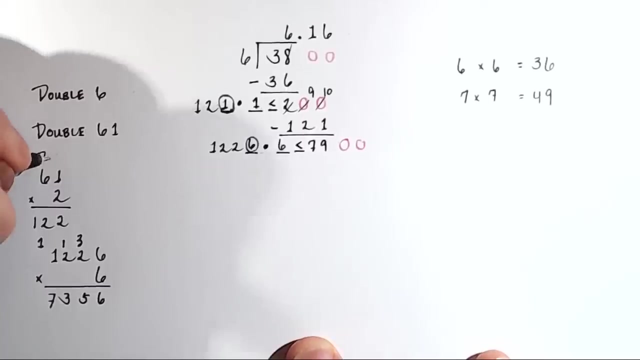 and a 6 here, And that means that 6 is the next digit in the approximated square root. So we'll go up here and put a 6.. Now, if you wanted to continue this process, you would double 6, 1,, 6.. 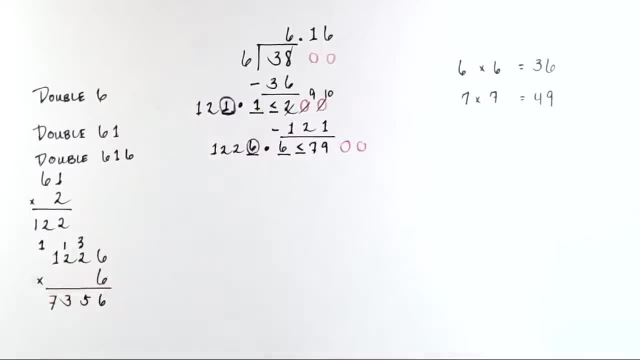 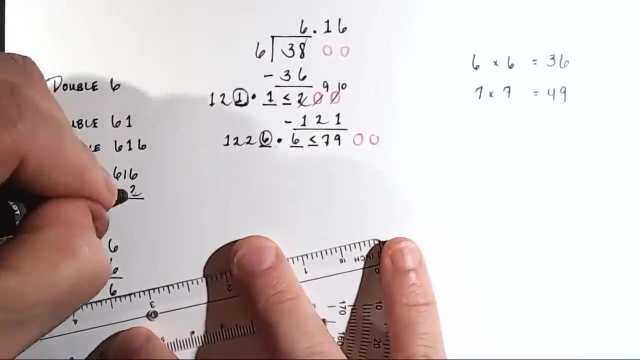 So when we double these numbers, we're taking the numbers without the decimal. So the next step in this process would be to take 6, 1, 6 times 2. And that would give me 12,. carry the 1,, 3, and 12.. 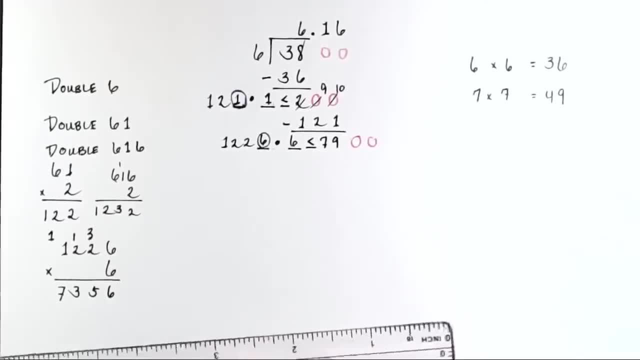 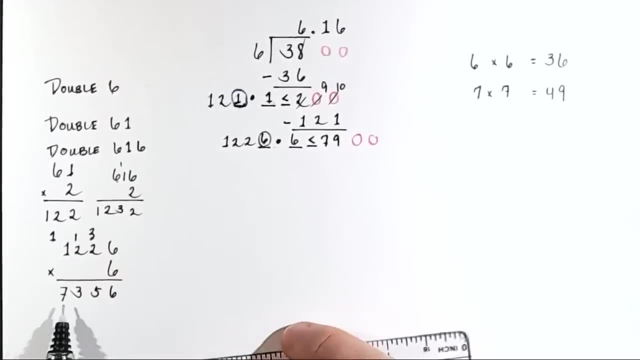 Okay, 1,, 2,, 3,, 2.. And we'll need that here in a moment, But we would take this. the next step in the process would be to take 7,, 3,, 5,, 6, and write it here. 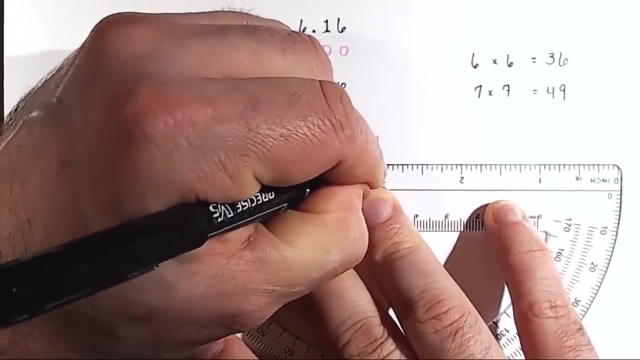 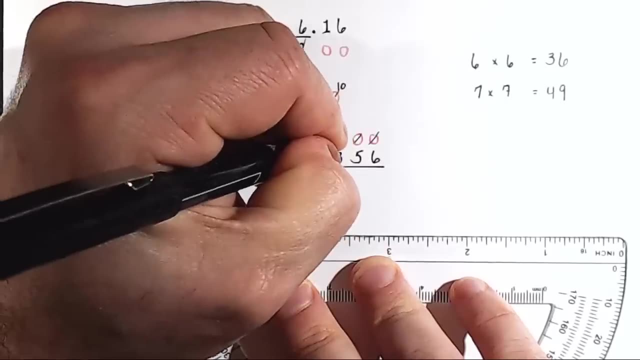 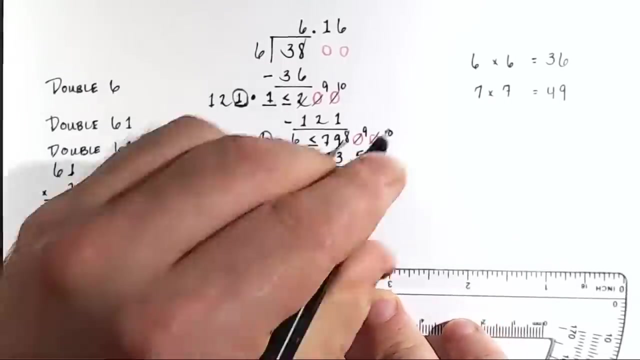 7, 3,, 5, 6.. Okay, if you, just if you wanted to continue this out for our purposes in math. we don't need to usually do that, but you could. Okay, so 10 minus 6 would be 4,, 9 minus 5 would be 4,. 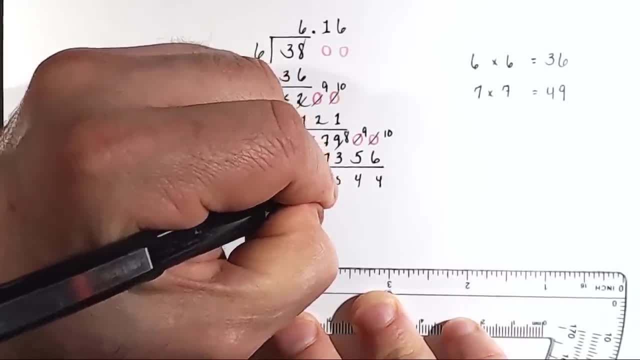 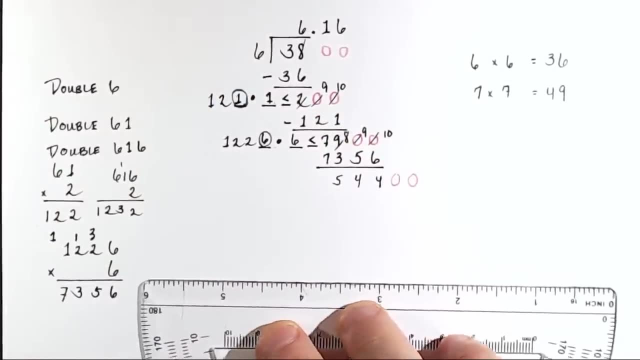 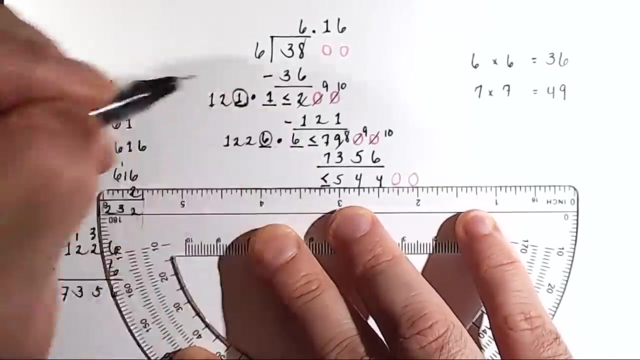 8 minus 3 would be 5, and that's it. So then we would bring down 2 more digits, And now we would be looking at 54,400.. And we would put less than or equal to symbol number. multiplication symbol number. 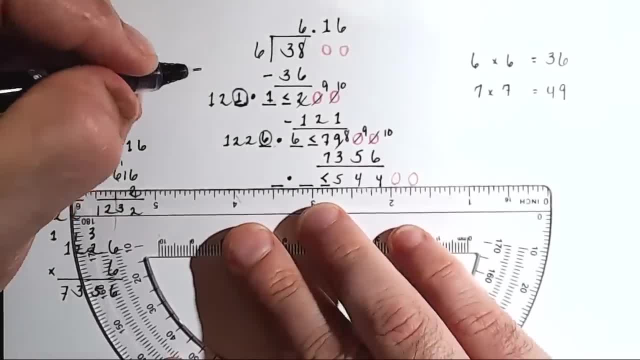 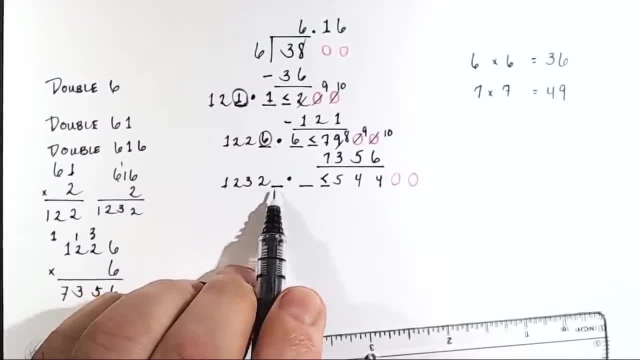 1,, 2,, 3,, 2.. 1,, 2,, 3,, 2.. 2, and we would be looking for that final digit. This is getting big right. It gets the problem itself gets big.